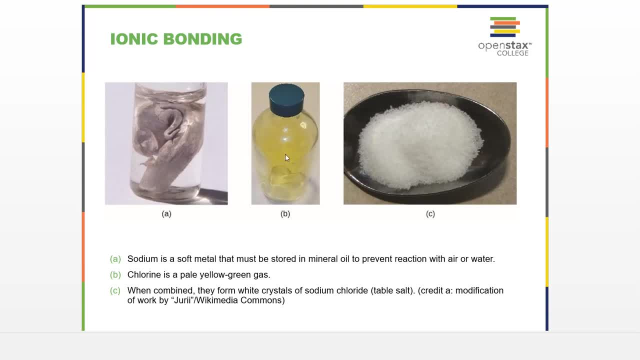 this nonmetal, in this case chlorine, to form sodium chloride, NaCl. NaCl table salt is this white crystalline powder. Chlorine is a yellow poisonous gas and sodium is a metal that is soft enough to cut with a butter knife. and 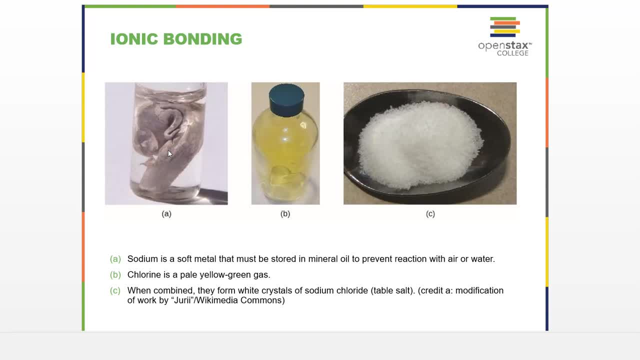 virtually catches on fire when it reacts with water. it's so reactive. So these two things are poisonous, if you will, and this is something that most people eat every day. And what is going on in an ionic compound, which we can recognize by the presence of a metal, is that sodium gives one. 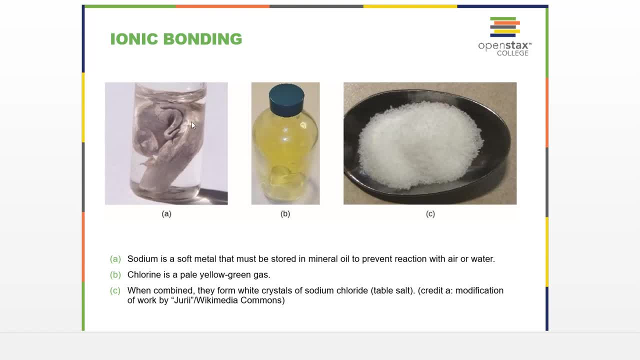 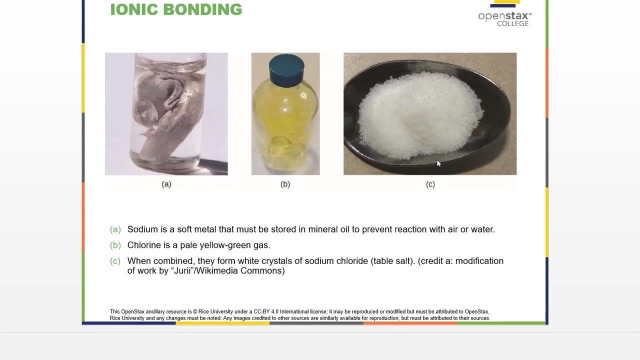 electron to the chlorine, sodium becomes positively charged, chlorine becomes chloride, which is negatively charged, And the positive ion and the negative ion are attracted to each other and we end up on the macro scale with table salt. Now at a deeper level, at the molecular level, what you end up with 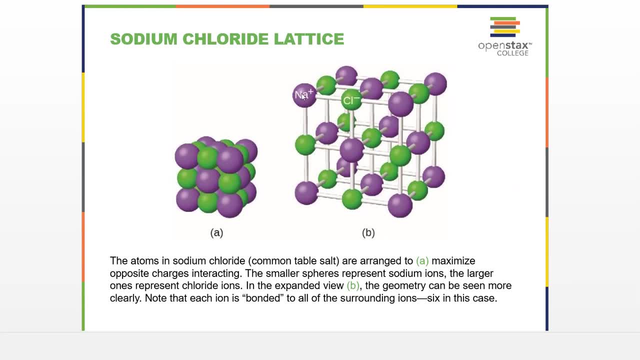 is these lattices, And here the purple balls represent sodium and the green balls represent chloride, And what you'll notice is that this sodium is completely surrounded by chlorides. It's got one behind it above, left, right, below and 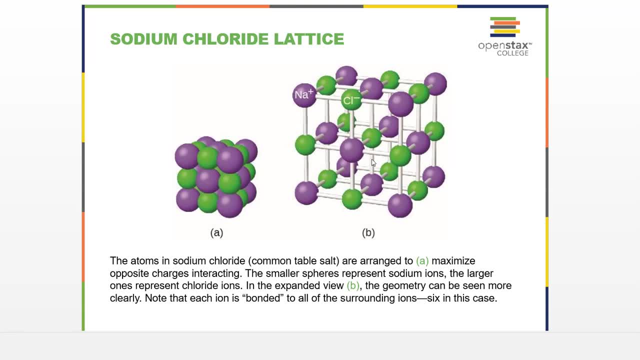 even in front of it, even though we can't see that lattice. And if we look at sodium, it's surrounded by chlorides. and if we look at chloride, it's surrounded by sodiums. Well, why is this the case? This is the case because 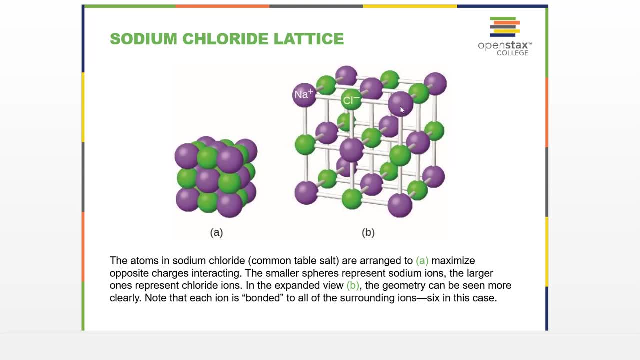 chloride is negatively charged, so it wants to be around as many positively charged things as possible. And sodium is positively charged, so it wants to be around all these negatively charged chlorides and you form this lattice And it turns out that if you want to separate these ions, which we'll 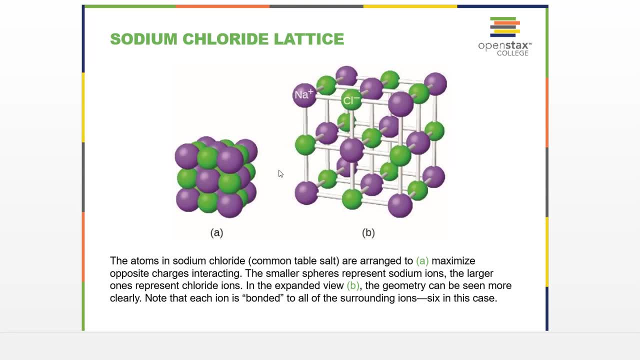 talk about a little bit later on in terms of something called lattice energy. it takes a massive amount of energy. The boiling point of salt is very, very high because it is a very stable arrangement of atoms in sodium chloride, which arises from the fact that you have positive ions next to. 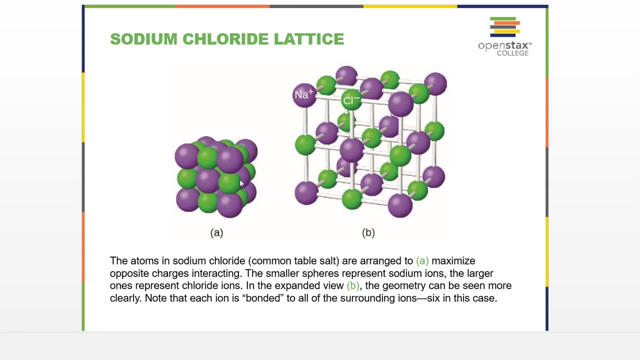 and interacting with attracted to negative ions in this lattice. Note that this is different than the macro viewer sodium chloride. this is what table salt looks like, But this is what the atoms, which you can, of course, see inside of table salt. this is how they're arranged. 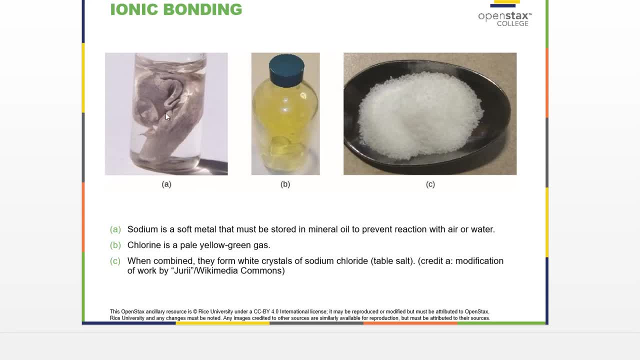 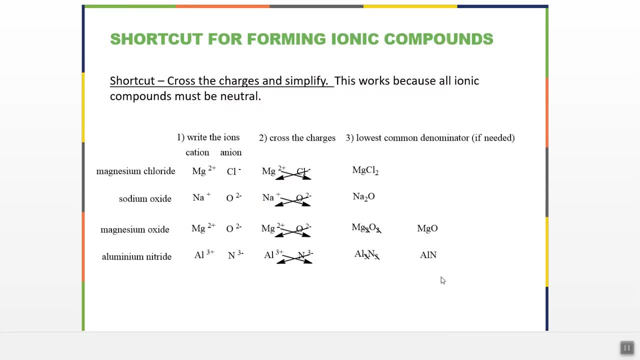 It's also important to note that table salt has very different properties from what it's made out of sodium and chlorine gas. As a reminder for ionic compounds- and this slide comes right out of chapter 2, we can form them by crossing the charges. Remember, we can identify ionic compounds because they 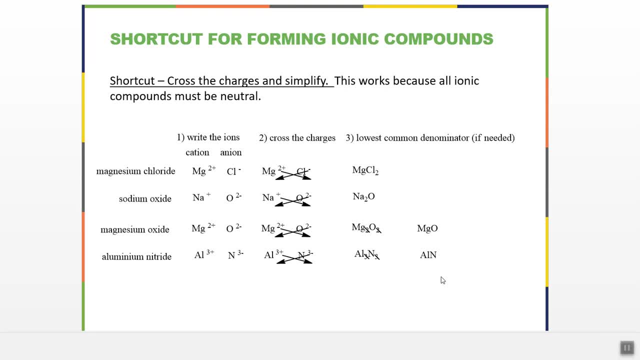 form between a metal and a non-metal and we can identify their structures by their charges. So magnesium is in 2a, so it forms ions that are 2+. chloride is in 7a, so it forms compounds that are minus. we cross the charges, we get MgCl2.. 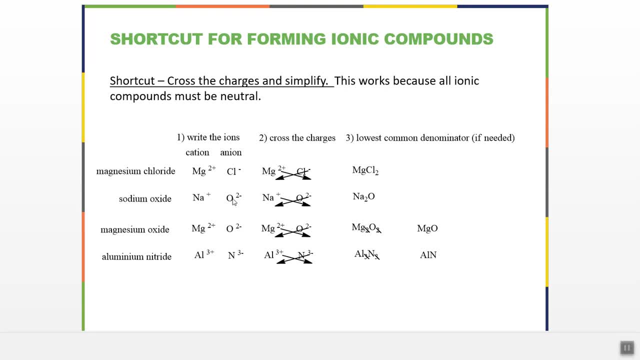 Sodium is in 1a, so it's plus. oxygen is in 6a, so it's 2 minus. we cross them. we get Na2O, Magnesium and oxygen. they're both 2, when they're both 2,, they have a. 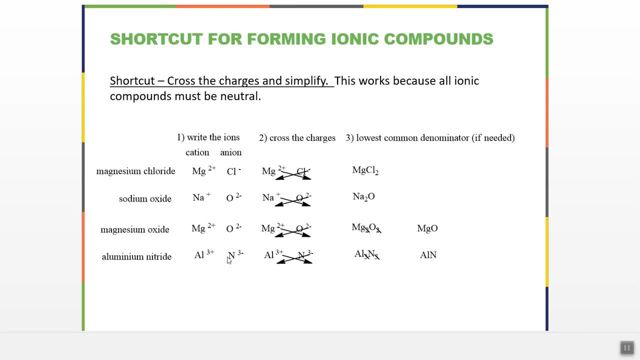 common denominator: we cancel out and we get MgO, in this case O2.. Aluminum and nitrogen, which are both 3, we cross them out and we get AlM. These rules still apply. They will come up again in this, in this chapter for. 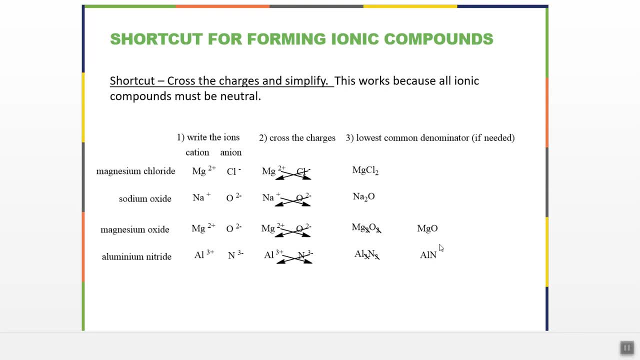 forming ionic compounds. The stable ionic compound has a neutral charge. It also contains a metal and a nonmetal or a polyatomic ion, So it's important to just remember the basic rules of ionic compounds. The new thing here is that 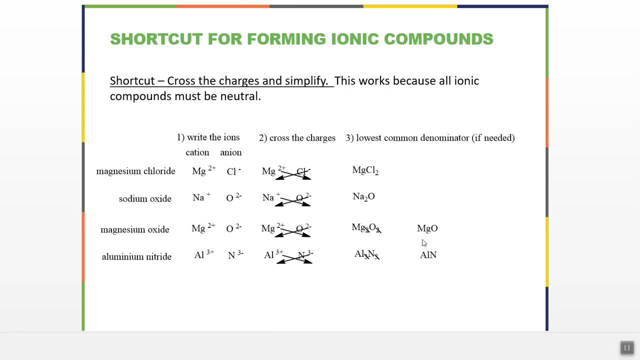 these ionic compounds exist in crystal lattices, where the positive ions are surrounded by the negative ion and the negative ion is surrounded by the positive ion And, as I mentioned a minute ago, in a few sections later we're going to look at lattice energy of ionic compounds to see how do they compare. So 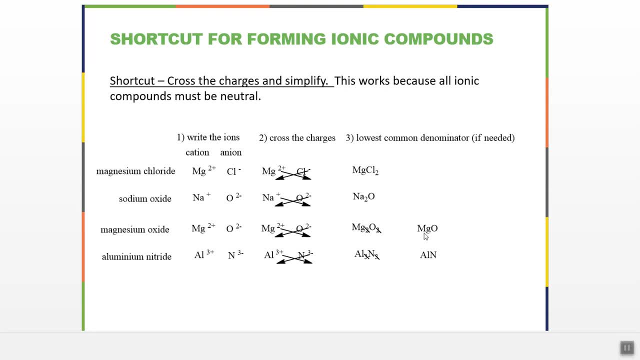 how does the melting point of the boiling point of sodium oxide compare to that of magnesium oxide? But next we want to look a little bit about covalent compounds. and covalent compounds are between two or more nonmetals and involve the sharing of electrons.